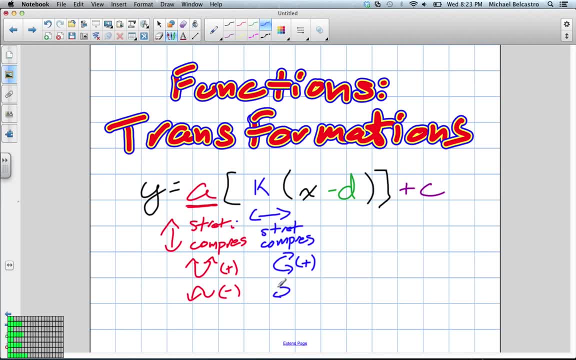 If you have a A root function, positive and negative, so horizontal flips okay, D deals with horizontal. So essentially, inside the brackets, everything's horizontal, Horizontal transformation. So it's just kind of opposite direction, though You would think of a positive term going to the left in a negative direction. 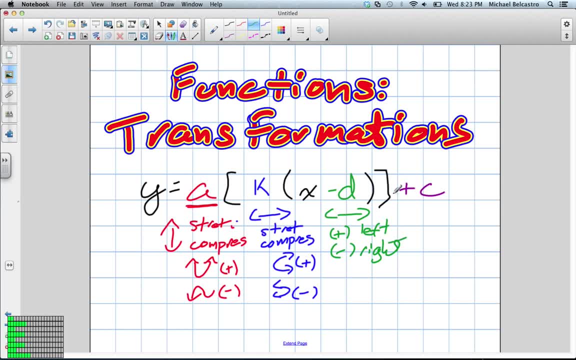 And a negative term going to the right. And then C is intuitive, In other words that it deals with vertical movements And positive is up and negative is down, which kind of makes sense for what we're talking about. So let's write down the function that they've actually given us to see if we can apply these rules to it. 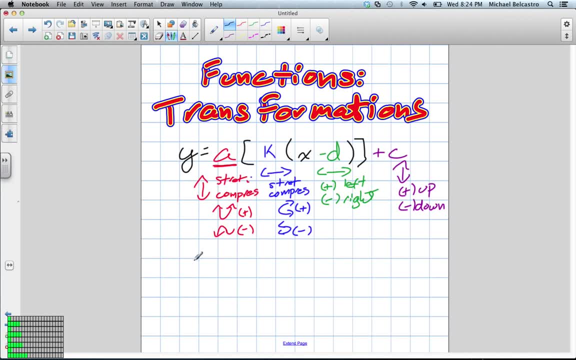 They've given us an absolute value function. They said that f of x is equal to 2, absolute value of x plus 3 minus 1, okay, So let's kind of zoom in here, Let's see if we can apply this. 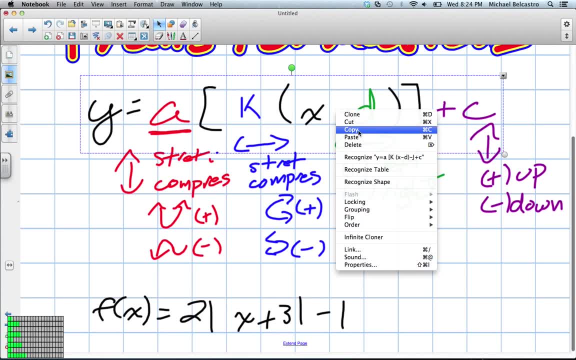 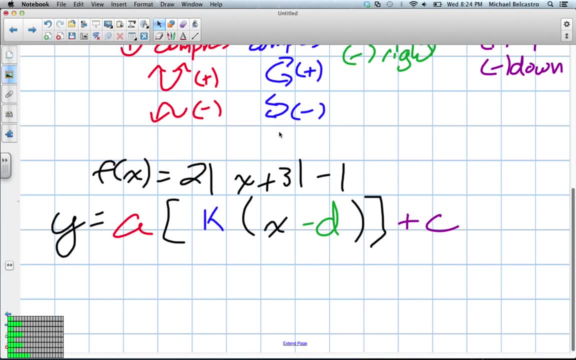 So copy, Then jump below it and see if we can. That's good, Okay, so in terms of these numbers corresponding to these variables, which do you think deals with which? Let's shrink it so it's a little closer. I think 2 would be A. 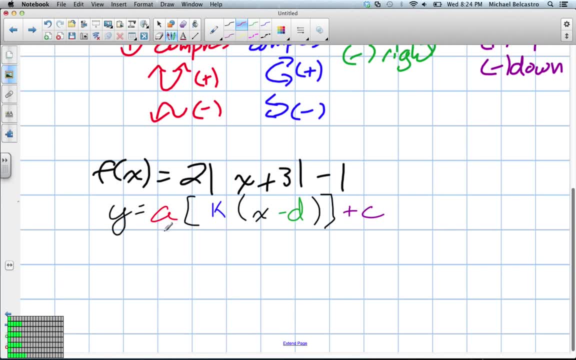 Yeah, that's right. Our 2 would be A. So, in other words, this is going to give us a. what Vertical stretch? Good, Vertical stretch, Good. So we're talking about vertical stretch, because A is equal to 2.. 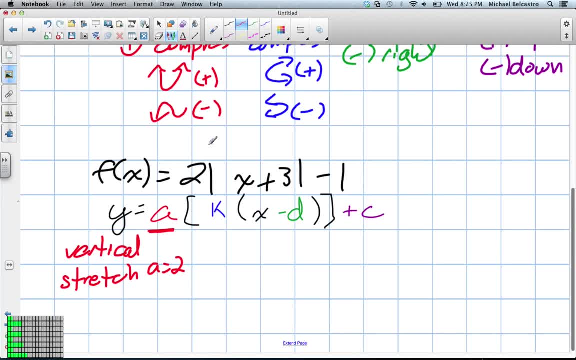 Okay, What else do you got? It goes to the left, right, I mean 3.. Yeah, okay, So that's going to be our D value, And because D is positive, we go in a negative direction. So we're going left 3 units. 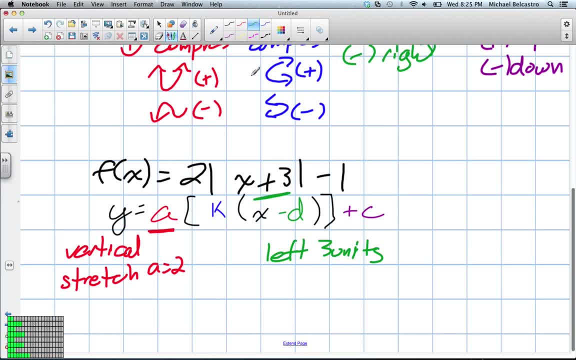 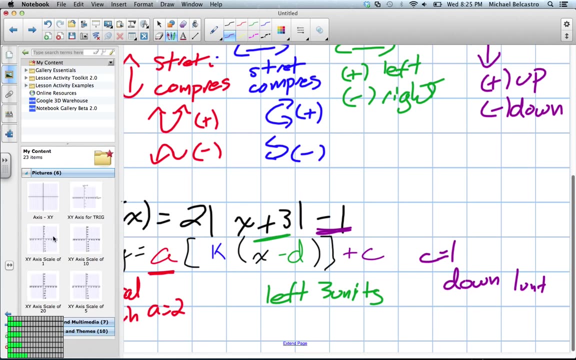 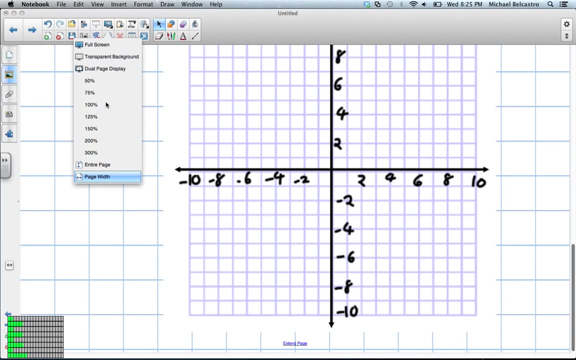 Good, There you go. And then what else? Down 1.. And then down 1.. Good, C is equal to 1.. So down 1 unit. Okay, So let's bring up our graph. Okay, That's good. 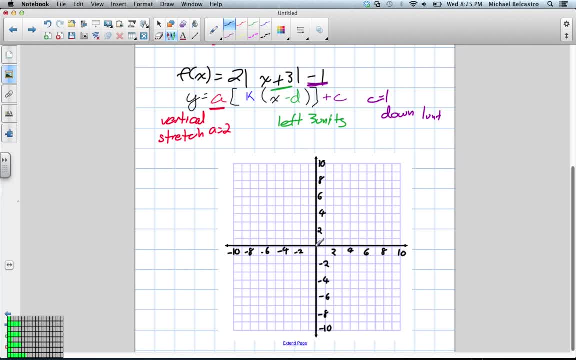 So we know that our Let's see if you know. What does a normal absolute value look like? Is it 1 over 1 up, 1 over 1 up, 1 over 1 up? Yeah, It's something like a positive sloped line and a negative sloped line. 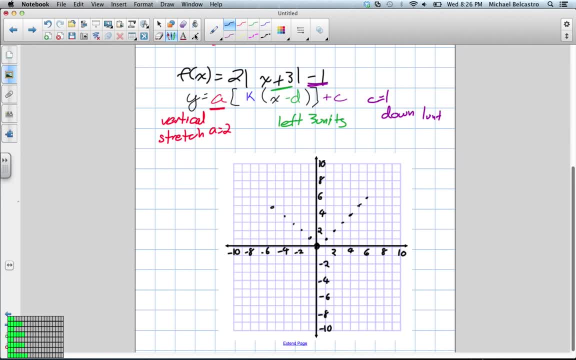 Okay, And the reason for this, and we'll draw these two lines, So that goes like that. So this is what we're talking about. transformations. We're talking about transformations from this. This would be. The original function would be: Y is equal to absolute value of X. 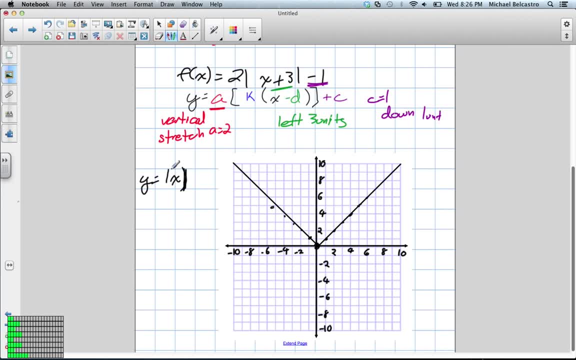 Not a straight line, And the reason it goes both ways is because if I put X at 2,, well, when X is 2, Y is 2.. When X is negative 2,, well, the absolute value of negative 2 is just 2.. 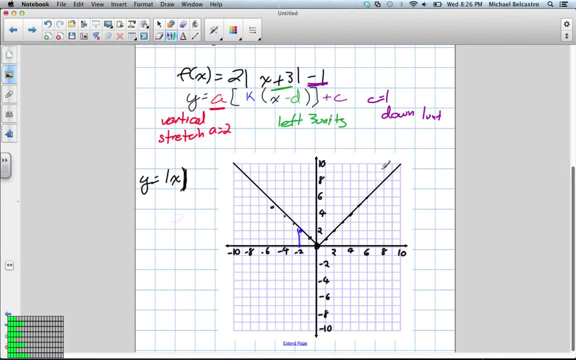 So we go to negative 2, Y is 2. And that's why they kind of follow that pattern. So what we're going to talk about is this original moving it around. So what we have here is: let's actually move that starting point. 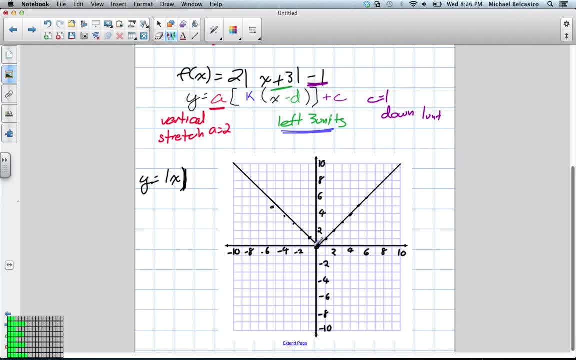 We know the starting point is going to go 3 units to the left: 1,, 2,, 3. And then 1 unit down. Okay, So because that's happening, we'll do it in, I guess, right here. 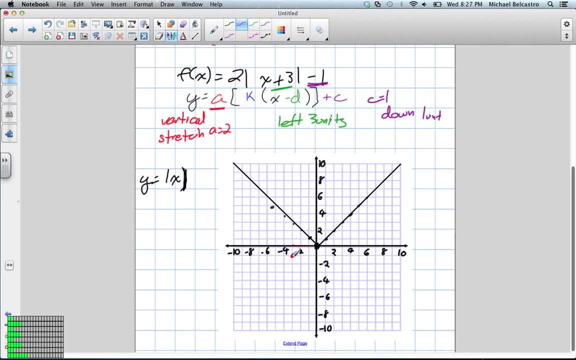 We've gone over 3 units: 1, 2, 3.. And down 1.. So this is now our starting point, And now I want you to think of it like this: This 2 in the front, think of it: whatever X value we have, we're going to multiply by that value of 2.. 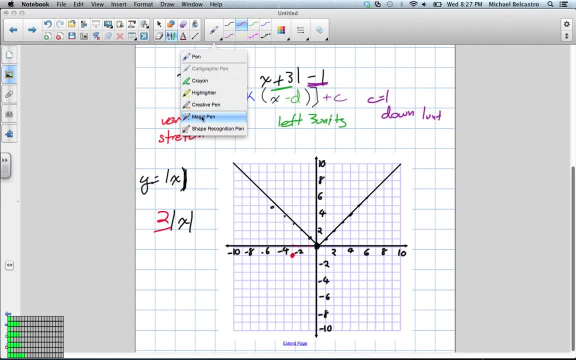 Okay. So normally we would go over 1, up 1. Over 2, up 2.. Over 3, up 3. But instead we go over 1 from here and up how many: 2. 2.. 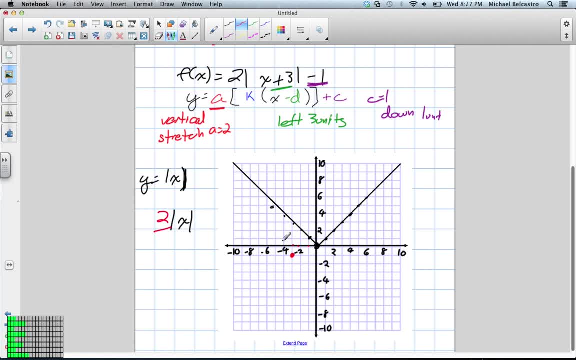 So it's going to look like it's being vertically stretched, pulled like an elastic band. you could say So: over 1, up 2.. Over 1, up 2.. Okay, Then we go over 2.. We normally go up 2.. 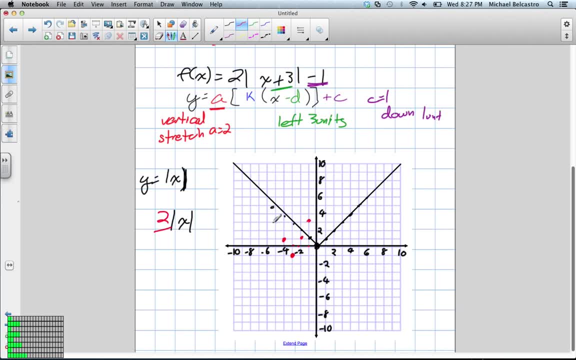 What do we have to go up this time? 4.. That's right. So we're still going to have straight lines. The only difference is they're going to follow a different- you could say slope- than they originally did. I think that's about right.